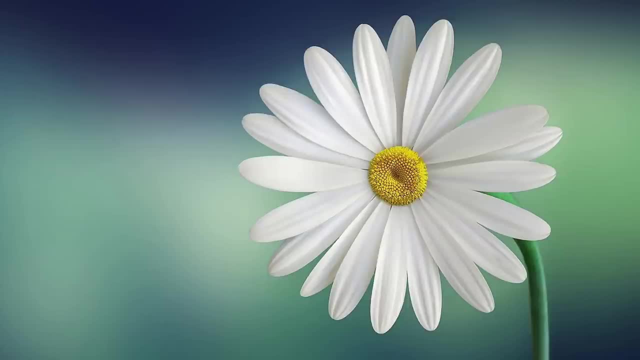 evolutionary context to help immediately understand what this is. But a computer doesn't have that same advantage. To an algorithm, the image looks like this: Just a few seconds later, the image looks like this: To an algorithm, the image looks like this: 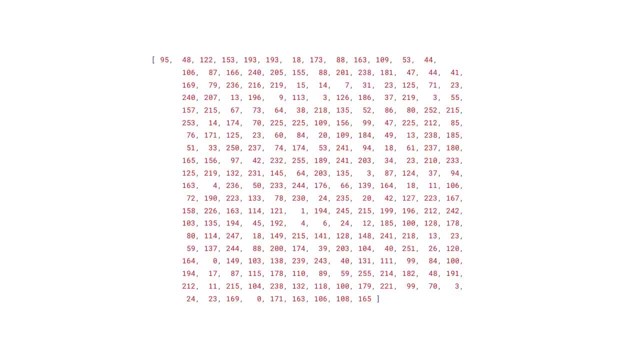 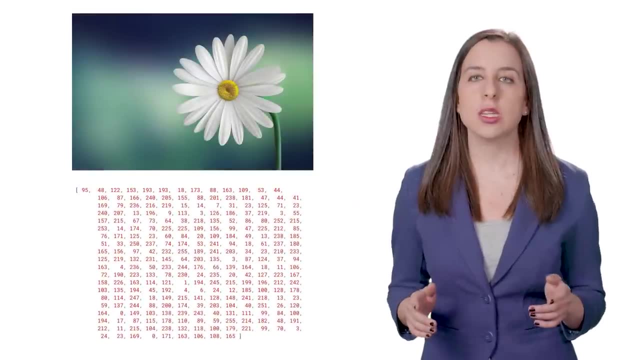 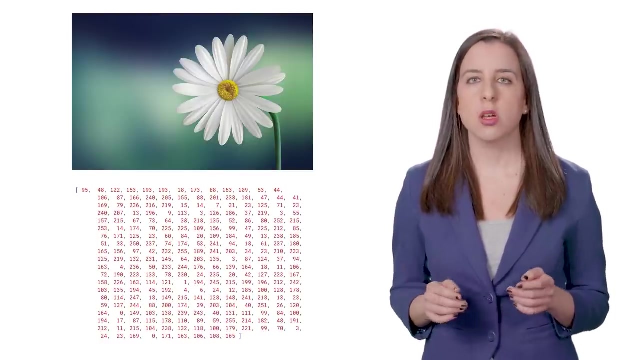 It's a massive array of integer values which represent intensities across the color spectrum. There's no context here, just a massive pile of data. It turns out that the context is the crux of getting algorithms to understand image content in the same way that the human brain does, And to make this work we use an algorithm very similar. 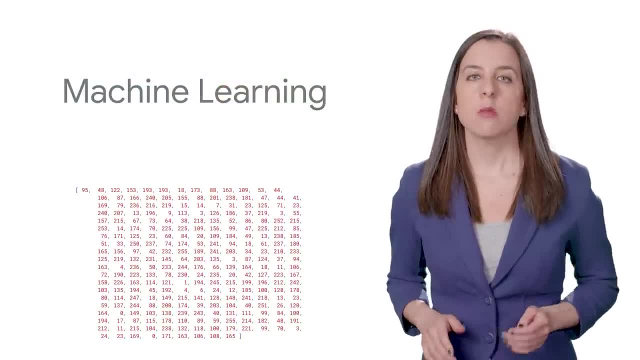 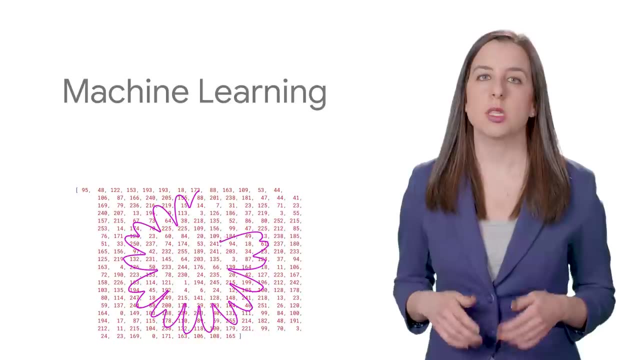 to how the human brain operates using machine learning. Machine learning allows us to effectively train the context for a data set so that an algorithm can understand what all those numbers in a specific organization actually represent, And what if we have images that are difficult. 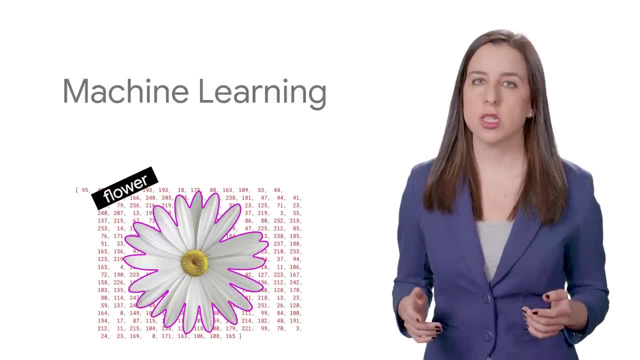 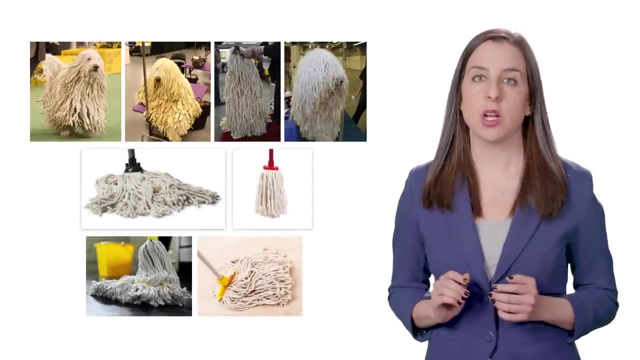 for a human to classify, Can machine learning achieve better accuracy? For example, let's take a look at these images of sheepdogs and mops, where it's pretty hard even for us to differentiate between the two. With the machine learning model, we can take a bunch of images of sheepdogs. 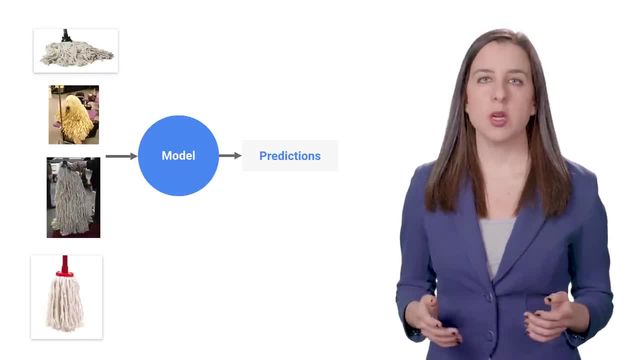 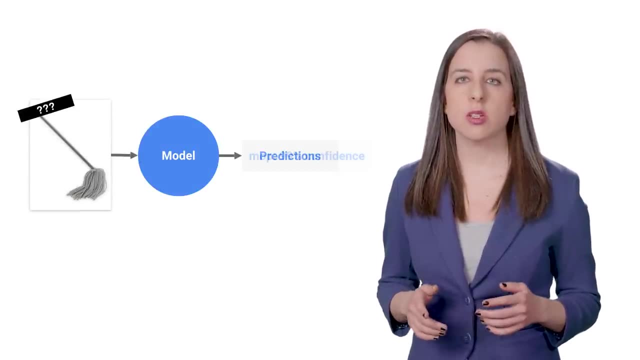 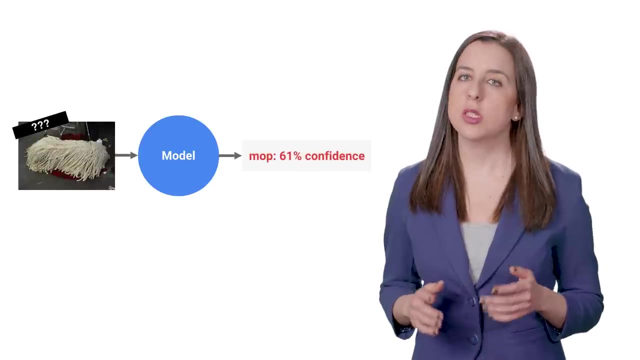 and mops, and as long as we feed it enough data, it will eventually be able to properly tell the difference between the two. Computer vision is taking on increasingly common and increasingly complex challenges and is seeing accuracy that rivals humans performing the same image recognition task. But like humans, these models aren't perfect. They do sometimes. 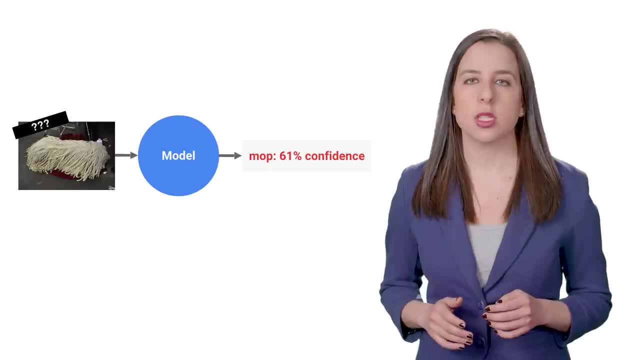 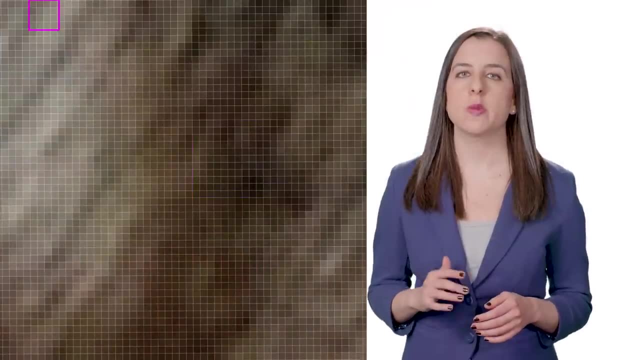 make mistakes. The specific type of neural network that accomplishes this is called a convolutional neural network, or CNN. CNNs work by breaking an image down into smaller groups of pixels, called a filter. Each filter is a matrix of pixels and the network does a series. 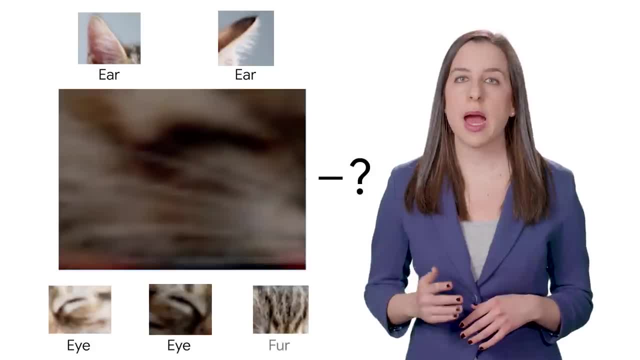 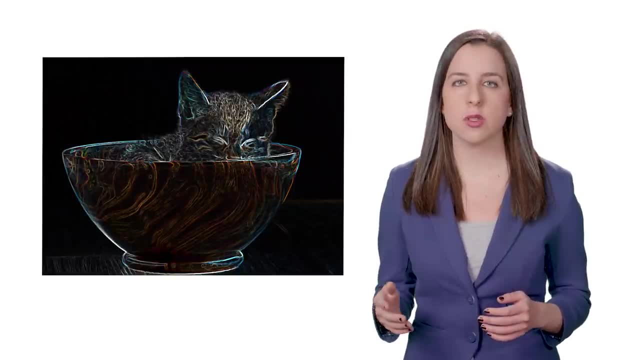 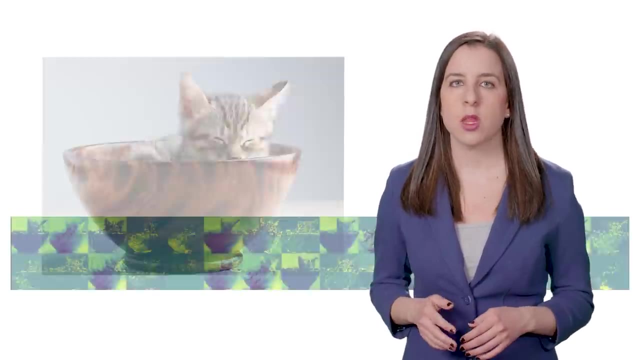 of calculations on these pixels, comparing them against pixels, to see what specific patterns the network is looking for. In the first layer of a CNN, it is able to detect high-level patterns like rough edges and curves. As the network performs more convolutions, it can begin to identify specific objects like faces and animals. 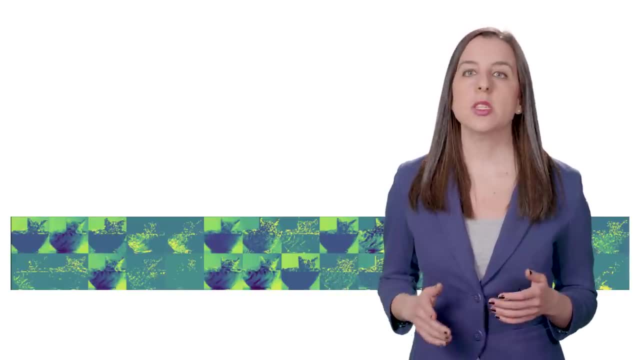 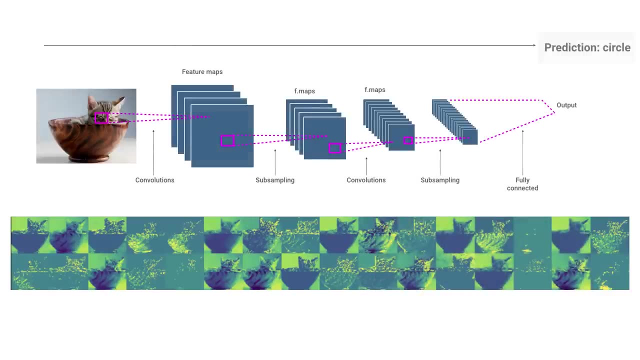 How does a CNN know what to look for and if its prediction is accurate? This is done through a large amount of labeled training data. When the CNN starts, all of the filter values are randomized. As a result, its initial predictions make little sense. 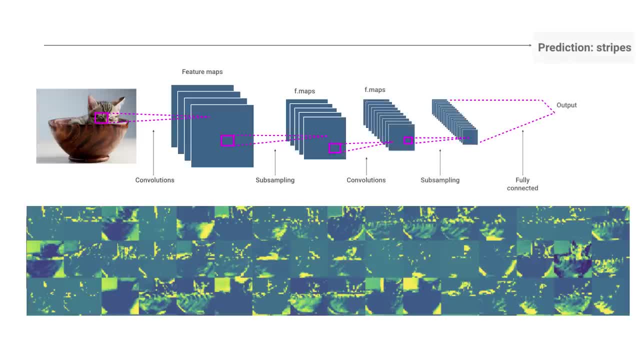 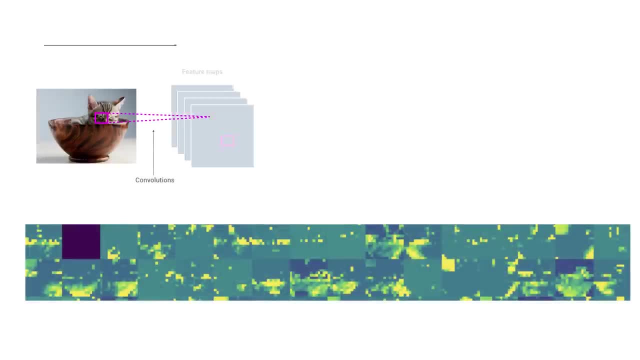 Each time the CNN makes a prediction against labeled data, it uses an error function to compare how close its prediction was to the image's actual label. Based on this error or loss function, the CNN updates its filter values and starts the process again. Ideally, 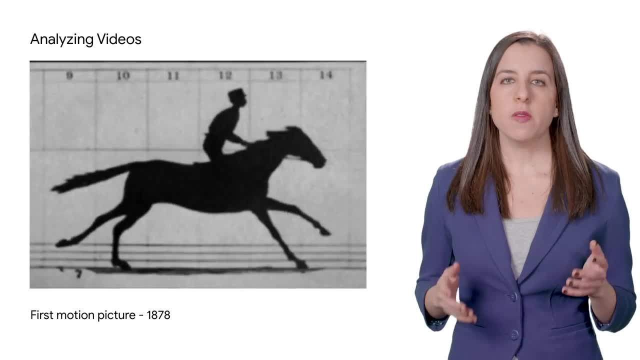 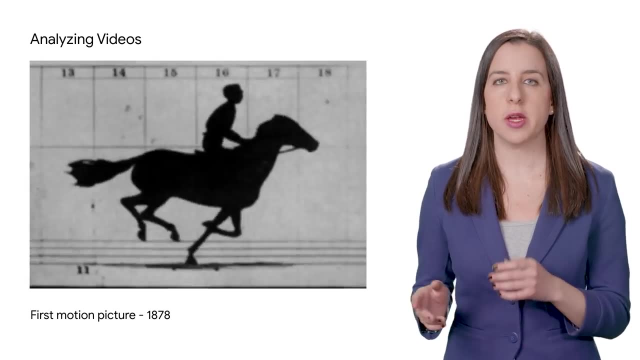 each iteration performs with slightly more accuracy. What if, instead of analyzing a single image, we want to analyze a video using machine learning At its core? a video is just a series of image frames. To analyze a video, we can build on our CNN for image analysis. 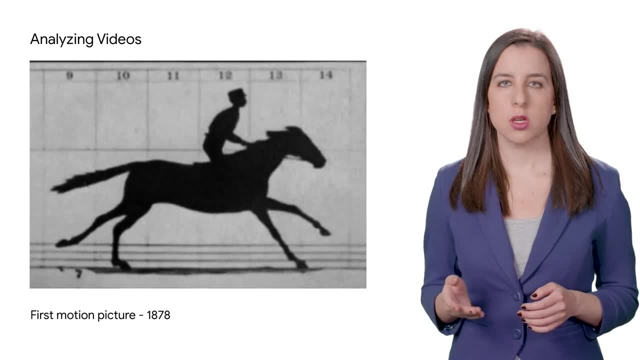 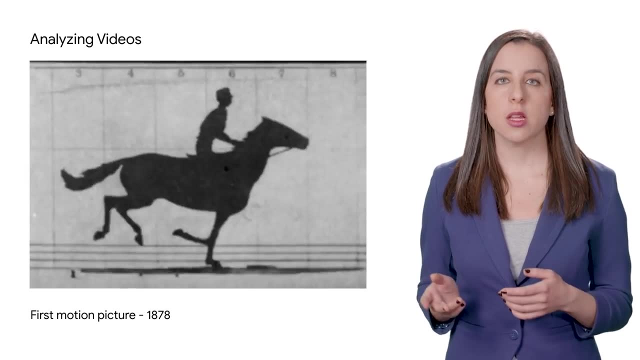 In still images, we can use CNNs to identify features, But when we move to video, things get more difficult, since the items we're identifying might change over time Or, more likely, there's context between the video frames that's highly important to labeling. 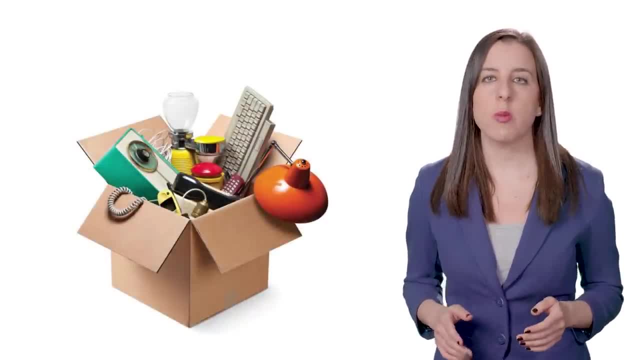 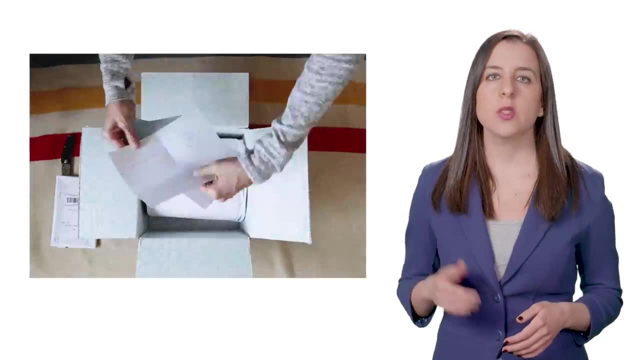 For example, if there's a picture of a half-full cardboard box, we might want to label it packing a box or unpacking a box, depending on the frames before and after it. This is where CNNs come up lacking: They can only take into account spatial features. 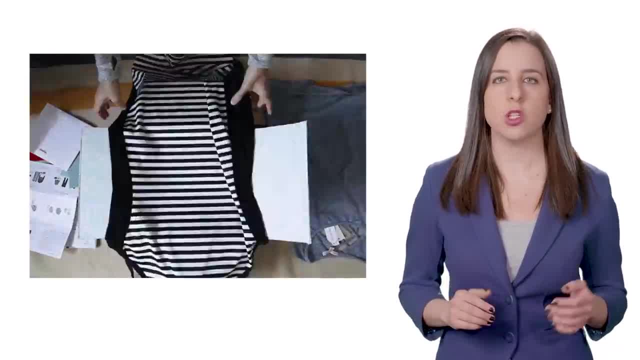 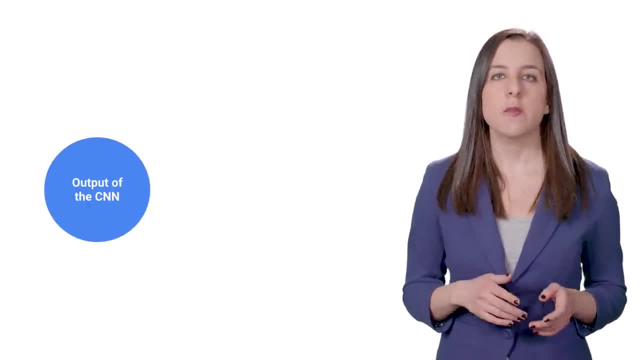 visual data in an image but can't handle temporal or time features how a frame is related to the one before it. To address this issue, we have to take the output of our CNN and feed it into another model which can handle the temporal nature of our videos. 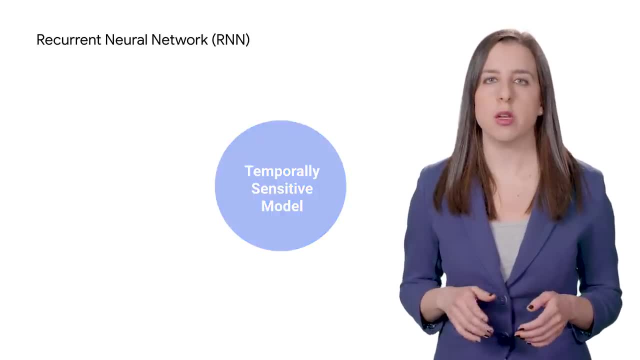 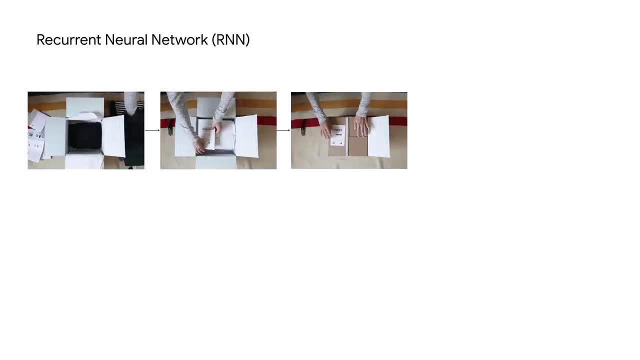 This type of model is called a Recurrent Neural Network, or RNN. While a CNN treats groups of pixels independently, an RNN can retain information about what it's already processed and use that in its decision making. RNNs can handle many. 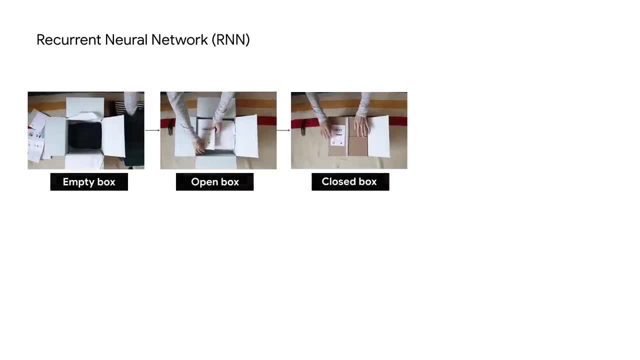 types of images, such as the image that we're looking at right now. For example, if we want to take a picture of an image, we can take a picture of the image that we're looking at right now. In this example of classifying videos, we'd train the RNN by passing it. a sequence of frame. 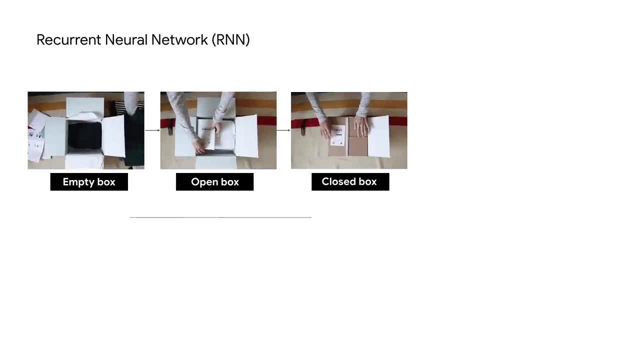 descriptions: empty box, open box, closing box and finally a label packing. As the RNN processes each sequence, it uses a loss or error function to compare its predicted output with the correct label. Then it adjusts the weights and processes the sequence again until it achieves a higher. 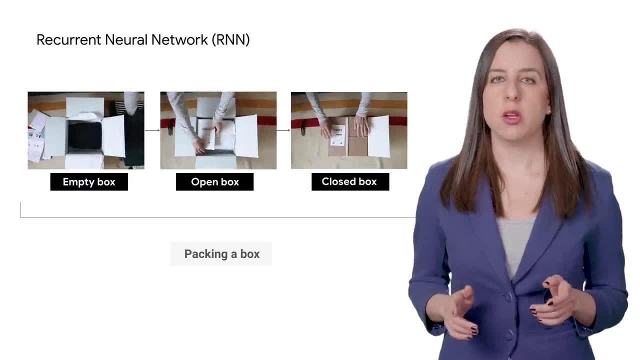 accuracy. The challenge with these approaches to image and video models, however, is that the amount of data we need to process in order to achieve a higher accuracy is very limited. The amount of data we need to truly mimic human vision is incredibly large If we train our model.